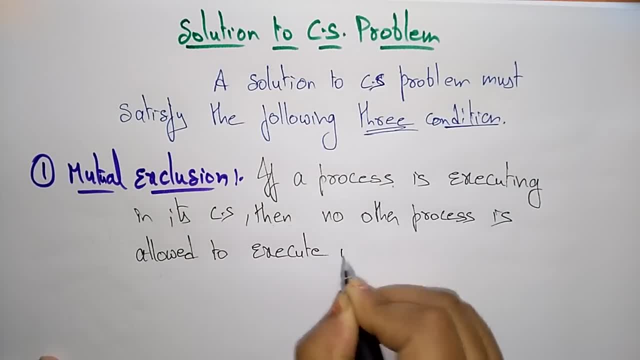 is executing in its critical section, then no other process is allowed to allowed to execute, so that you call it as a mutual understanding between the process. so, whatever i said it, the people wants to see, the group of people wants to see the movie. okay, p1, p2, p3- the three process. 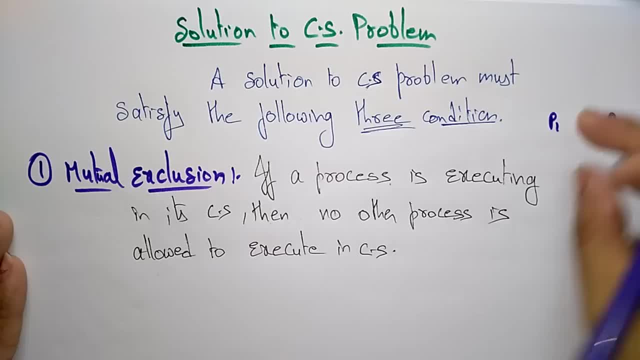 wants to see the movie, so the p1 will. some group of people are informed as a p1, p2, p3, so they will understand to means one agreement means the first. the p1 will want to watch next p2, next p3, so there is an. 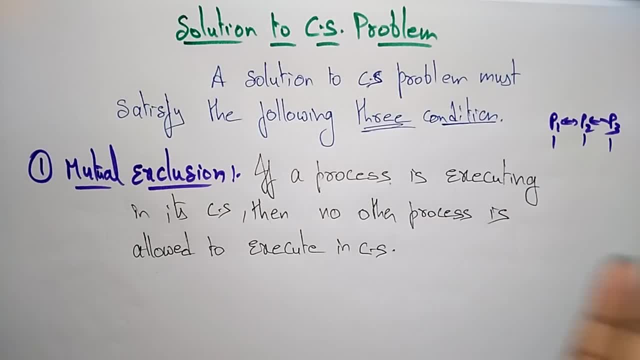 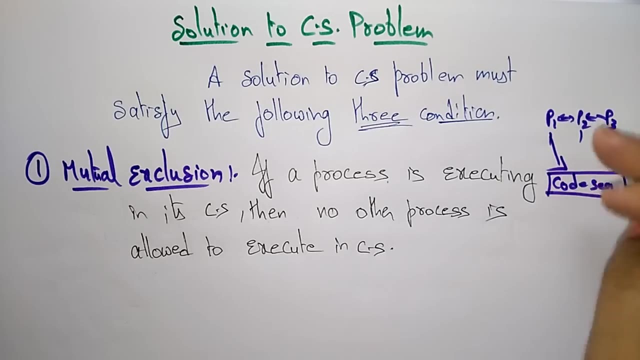 understanding between those process, those people, so that you call it as a mutual execution. so whatever the process is executing in its suppose p1 wants to use the code segment that is the amphitheater it wants to use first. so whenever it enter into code segment the p1, that is a critical section. no other process allowed to execute means these. 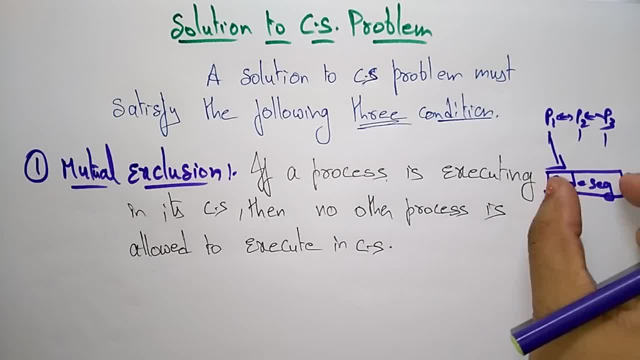 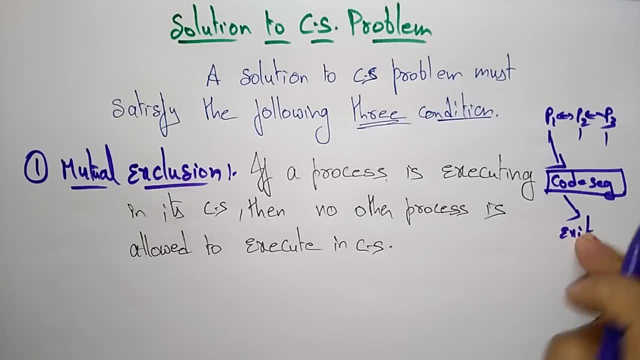 people are not allowed to enter into this amphitheater until they watched the completed the movie, so after that they will report, report it as exit. so whenever this p2 sees the exit, then next p2 will enter and you have to remember that, whatever the process that are there that the cpu wants to execute, 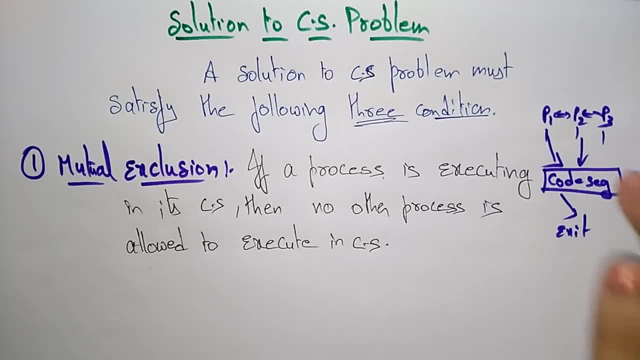 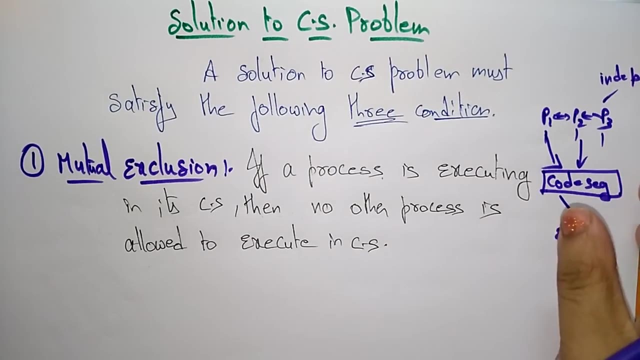 every process is, there is no need to enter into critical section because only the process that are using the shared variables, those process will enter into critical section. suppose the p3 is independent. those p3 people wants to see the movie at their home? okay, they don't want to use the amphitheater. 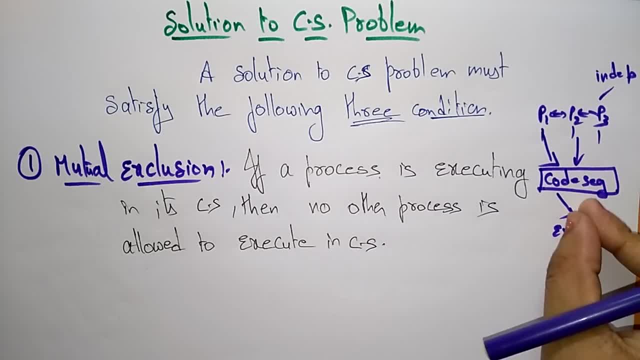 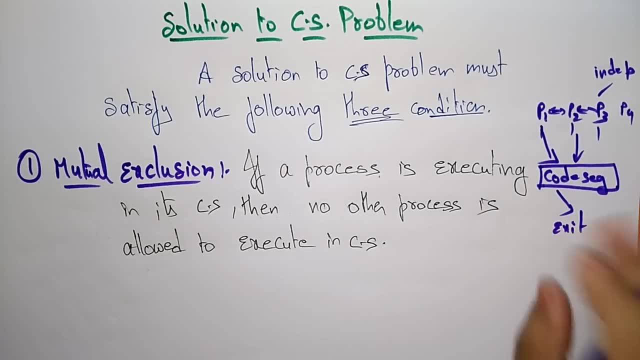 because this is independent, so they don't you enter into critical section, they will go and watch that movie at their home. okay, next p4 will enter into code segment, so like that. so there is no compulsory that all process will enter into critical section, only those process that user, the 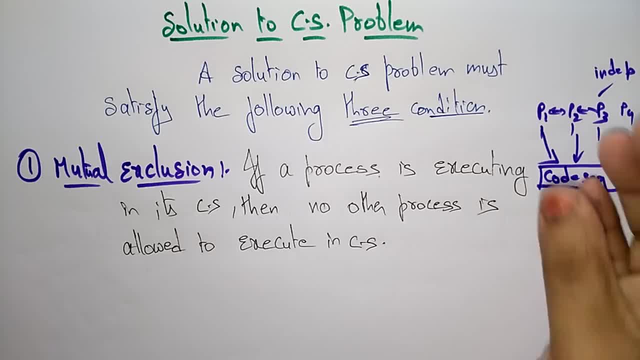 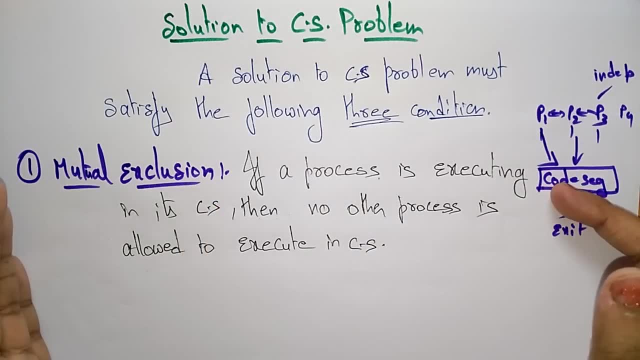 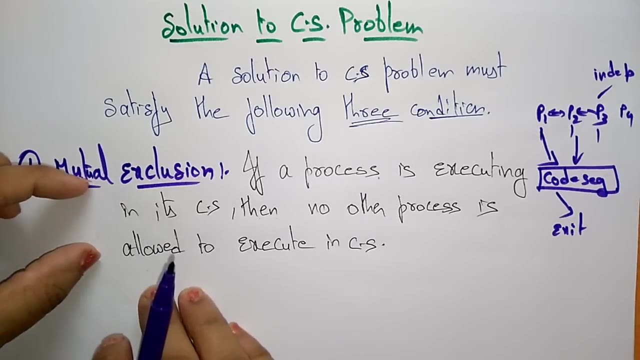 shared variables. okay, those control variable will enter into critical section. so i hope you understand. mutual exclusion means if one process is executing in its critical section, then no other process is allowed to execute in critical section. so the first condition is this: that it's a mutual exclusion has to be followed. and next, these three conditions써 compulsory means, if you take at least two conditions or to be satisfied, whatever the process that is entering into critical section. so the first condition, which is particular to the cut, the códigoRL, which here we have to use: communication sit interesting, non non confronting, tentative client body in cosmetics worden become strong, limited by the purpose that he or she gets impossible soldier. here we have to explain to you some things. the purpose of abuseвол, what neste capacity? initial task you to discover that the process is to reduce your father, renovation of the burning process, so that you can, you can clearly understand in criticism. so i hope you understand mutual exclusion means if one process is executing in critical section. 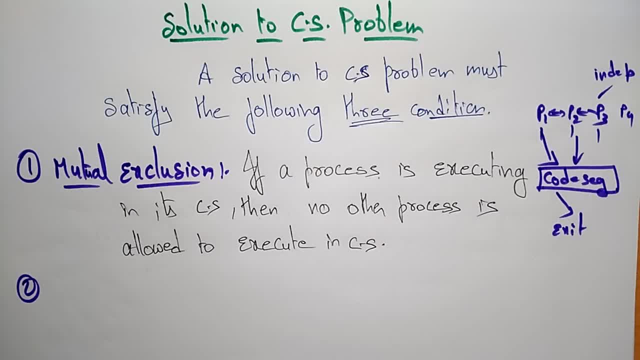 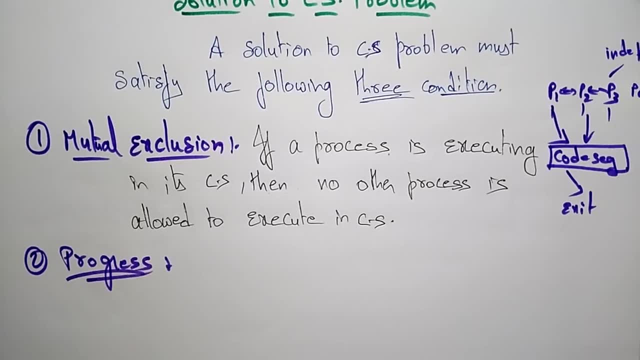 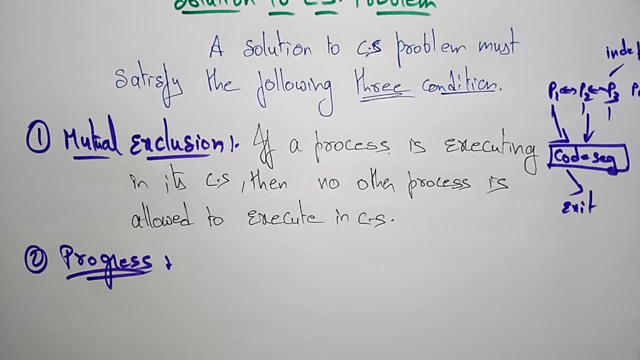 First is mutual exclusion is compulsorily, it has to be satisfied. Next is the progress. So what we mean by progress? A progress means if no process is in critical section, then no other process from outside can block it from entering the critical section. 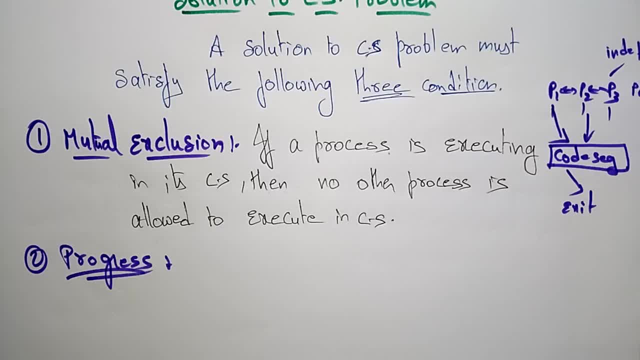 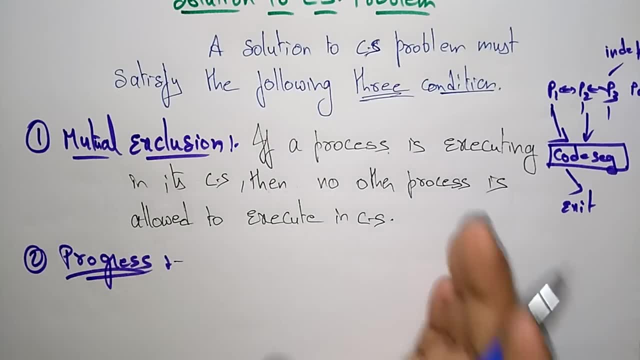 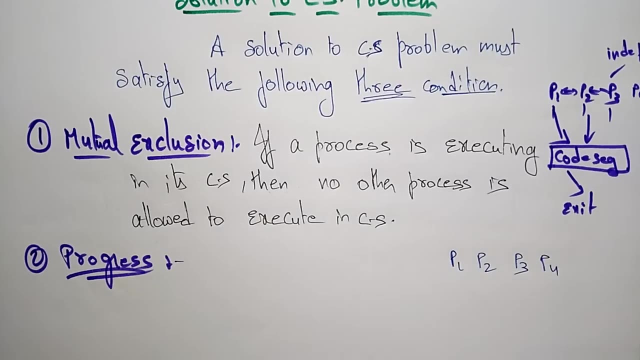 So what it means. So here he is saying that no process will enter into critical section, then no other process from outside are allowed. So exactly what it means. Suppose those process that wants to enter into critical section, suppose here P1, P2,, P3, P4, four process are there. 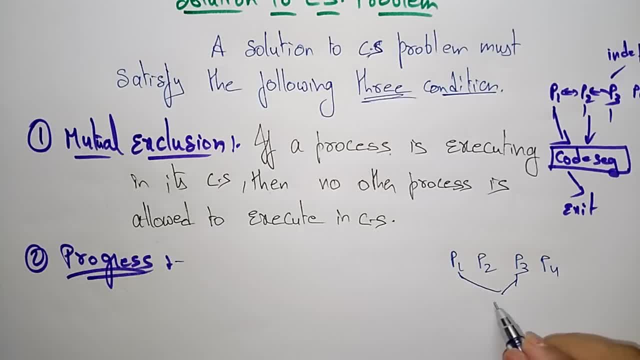 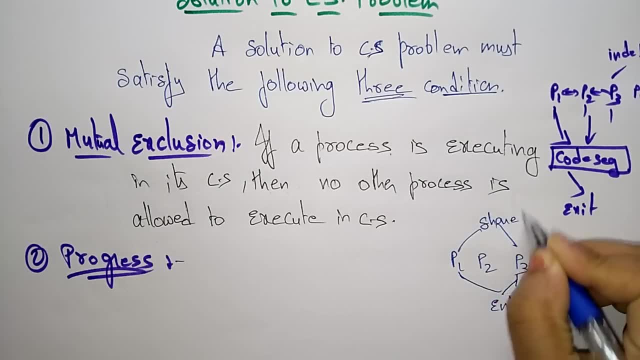 Only P1 and P3 want to enter into critical section. wants to enter critical section. Why only these two process? Because those are using the shared resources. They want to see the movie in the amphitheater because they are using the shared resources. 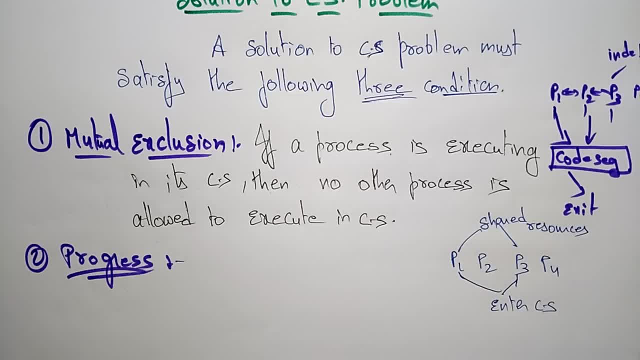 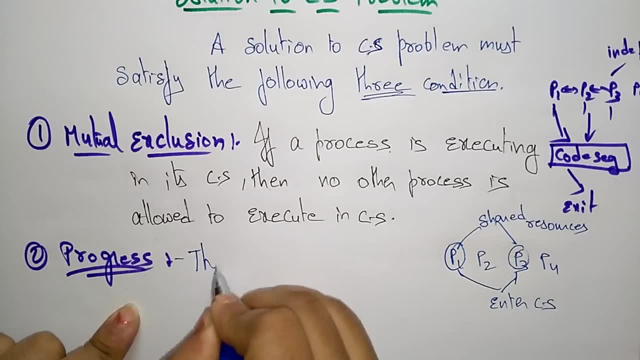 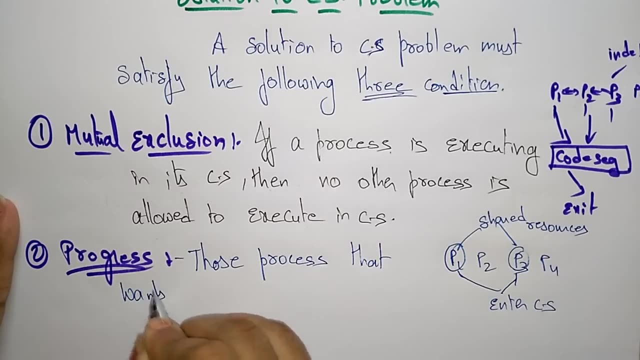 And P2, P4 are independent. So here progress means those process that wants to let me write that, those process that wants to enter into critical section. that has to be allowed. Only these two process has to be allowed, So that has to be allowed. 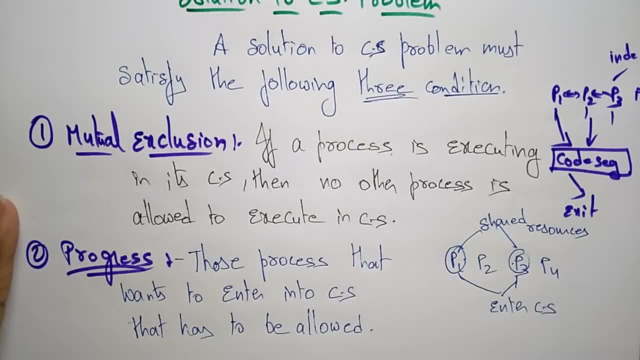 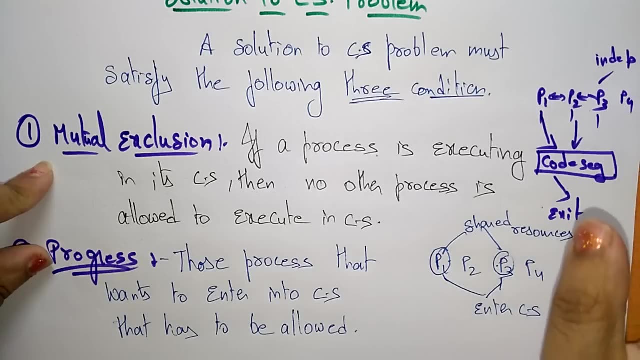 So that you call it as a progress. So first condition is a mutual understanding will be there from each process. Okay, So whether it is a independent resources or whether it is independent process, whether it is a cooperative process, some understanding should be there. 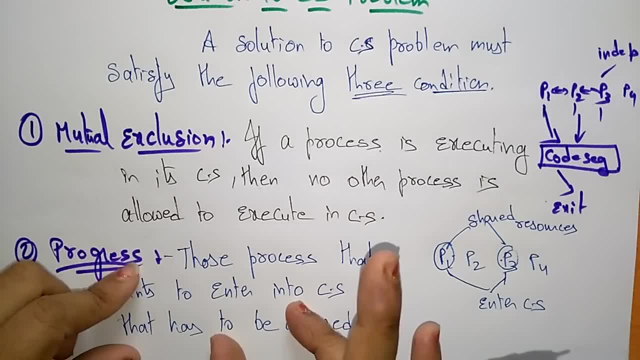 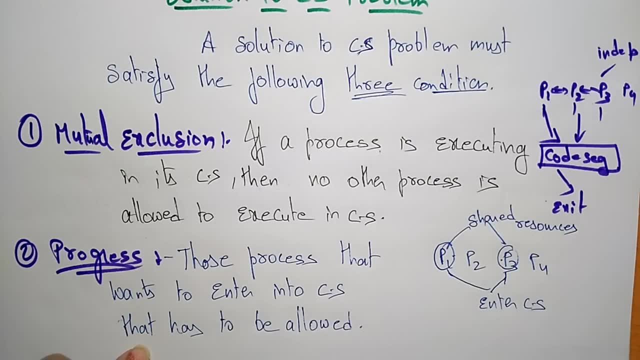 So one process is entering, no other process are allowed, Then progress means Don't send all the process into critical section. Those process that want to enter into critical section, that has to be allowed into critical section. So that is second solution. second condition: 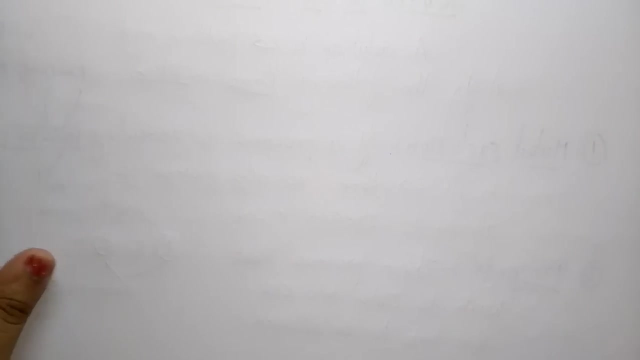 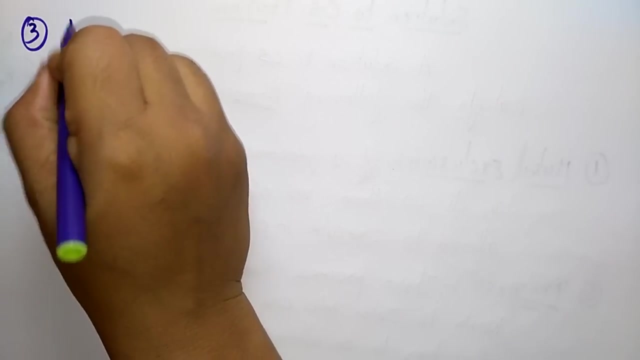 And the third condition. so this third condition is not that much of mandatory. Whenever it uses it, that problem is there, then you can go for this third condition, That is a bound weighting. So these three are the conditions that. 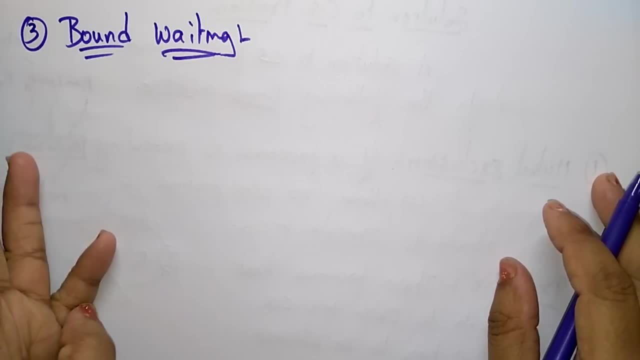 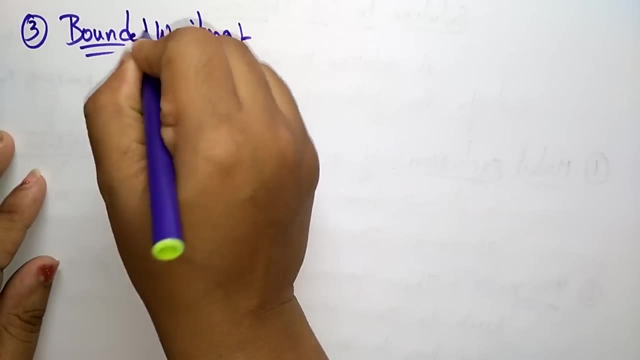 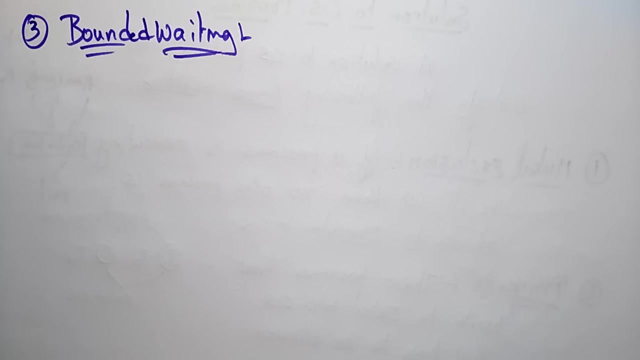 Which solves the critical section problem. So first they check the mutual exclusion, Next they will check the progress, Next bound weighting. So what is this bounded weighting? Let me write bounded weighting. This bounded weighting means suppose, after a process, make a request for getting into critical section. 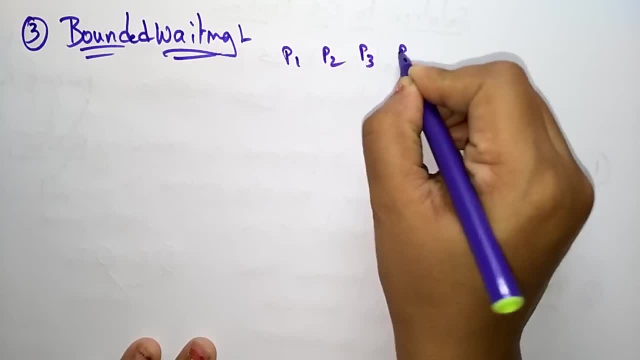 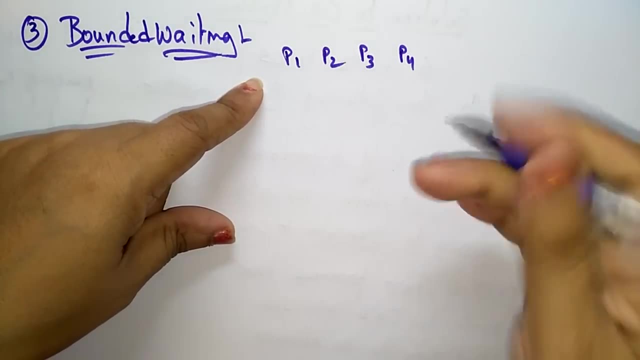 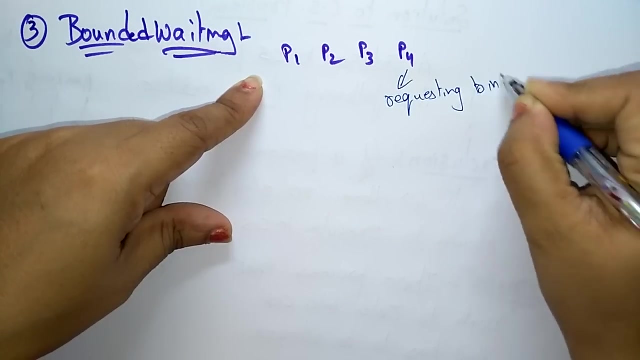 Here let me take P1, P2, P3, P4 process. are there? Okay, So after a process makes a request for getting into critical section, This P4 requesting let me take requesting to enter enter into critical section. 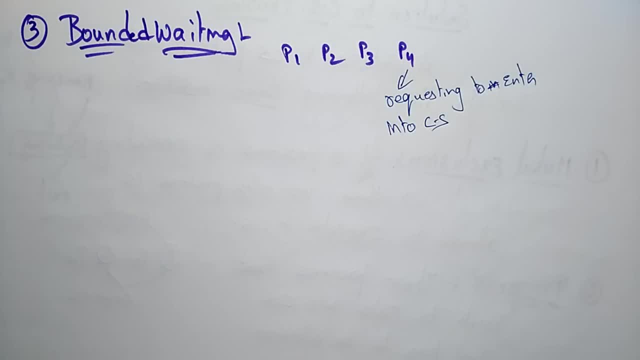 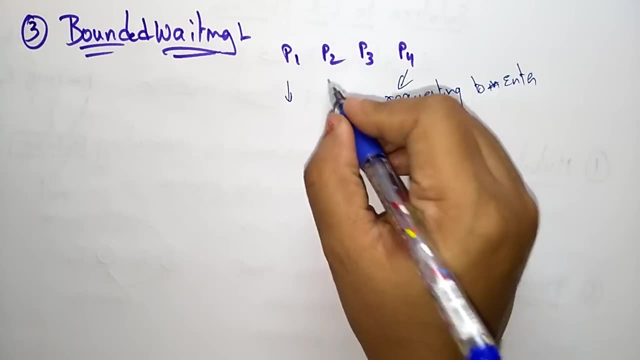 There is a limit for how many other process can get into the critical section Before this process request is granted. So first P1 is executing, P2 is executing. Again P1 wants to be execute, Next P2 want to execute. 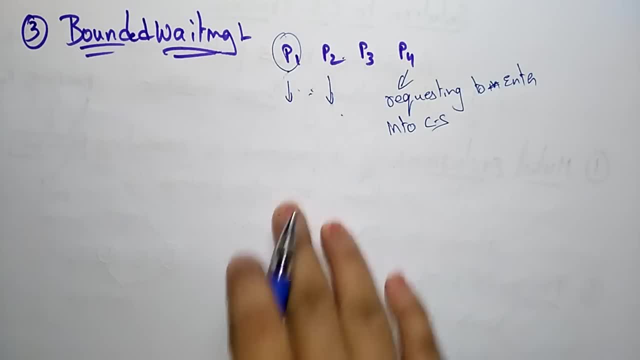 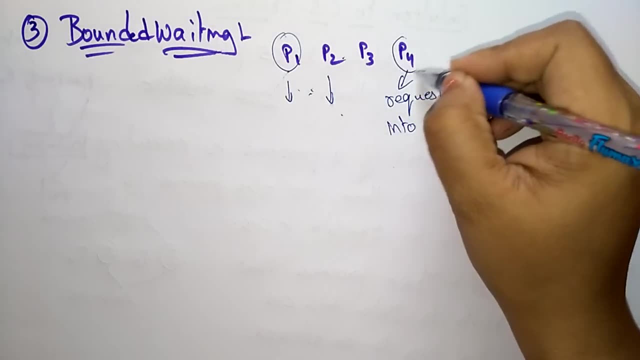 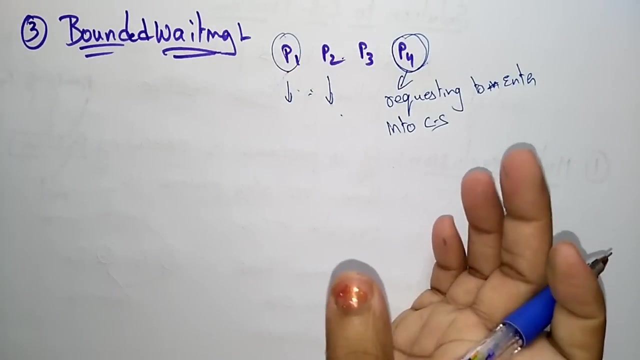 Means like that. it is continuing The process are entering critical section and exiting, and entering, exiting. like that, The process continue like that. But P4 chance was not coming. So that's why, if you want to solve this problem, we are using this bounded weighting concept. 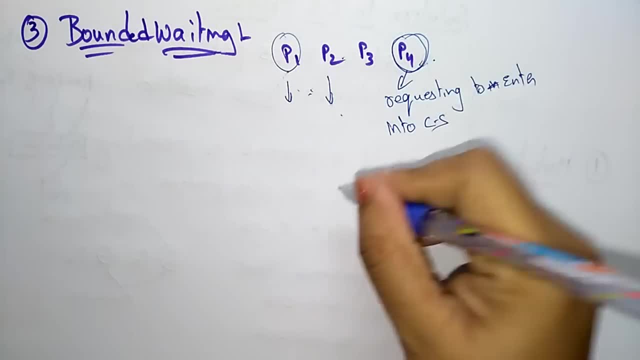 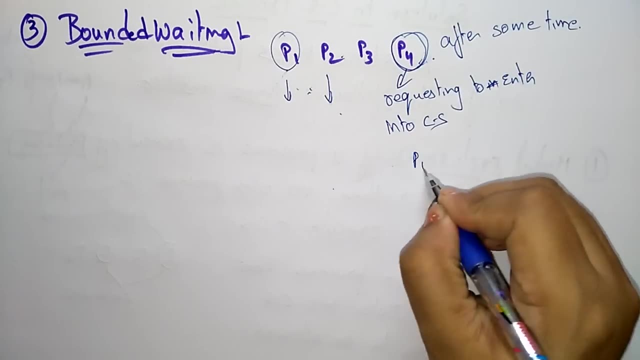 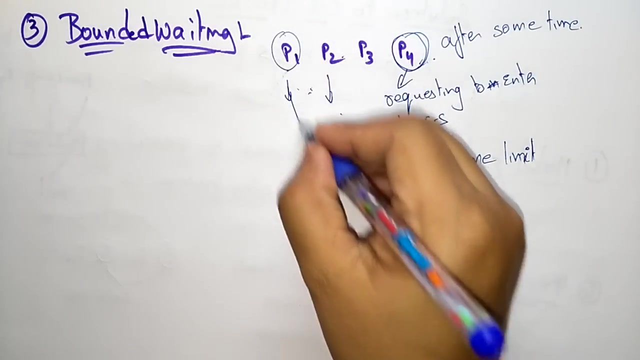 The bounded weighting concept means P1 is requesting to enter into critical section after some time, Means it is Setting one time limit. P4 is setting some time limit, So before that time limit, whatever the process wants to enter into critical section, they can enter.